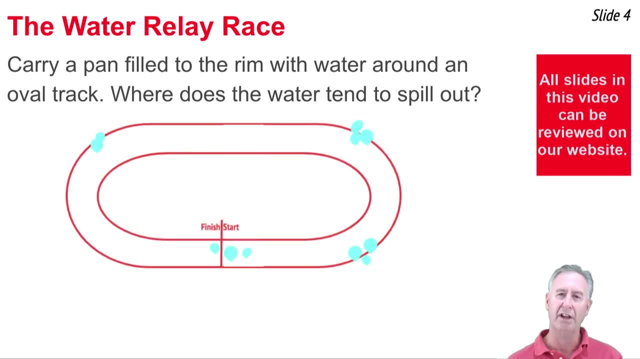 You would notice, the water falls out at the start line, at the finish line and at the turns. That's what you observe time after time. Every student observes. Every student observes One of these things. that's where the water spills over the rim of the container. 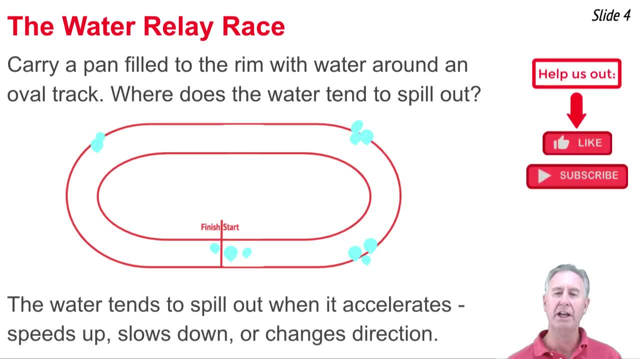 Why does this happen? Well, the water spills over the rim of the container. whenever you try to accelerate the water, whenever you try to change its state of motion or its velocity, It does it upon starting at the start line. The water wants to stay right there at the start line as you speed up the pan. 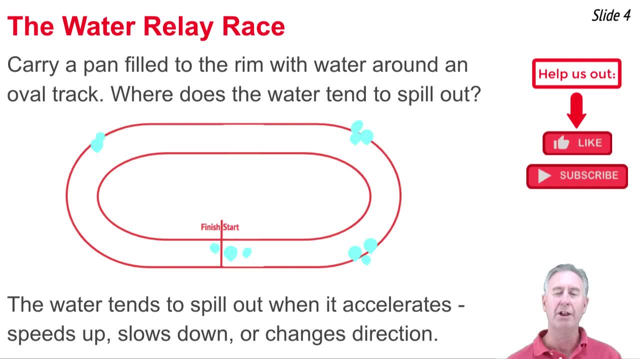 It does it at the finish line. When you try to bring the pan to a stop, the water tends to keep going. It spills over the front rim of the pan and it does it on the turns when you try to change the direction of the water. 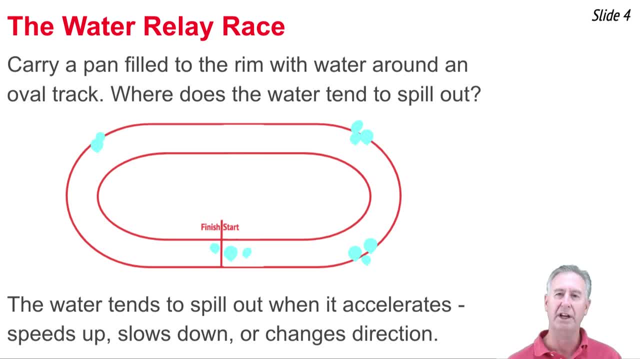 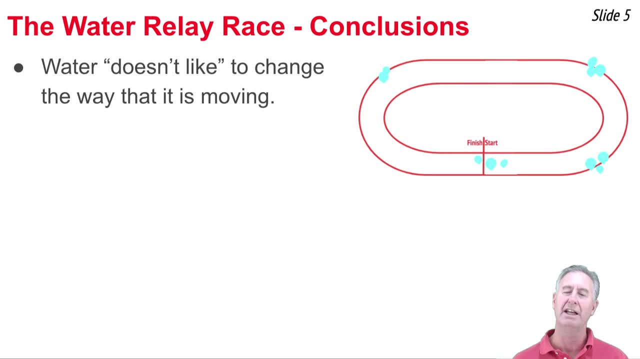 Water has this tendency to spill out whenever you try to accelerate it. So what conclusions does this lead us to about water? First, it leads us to the idea that water doesn't like to change the way that it's moving. It likes to keep on doing whatever it's doing. 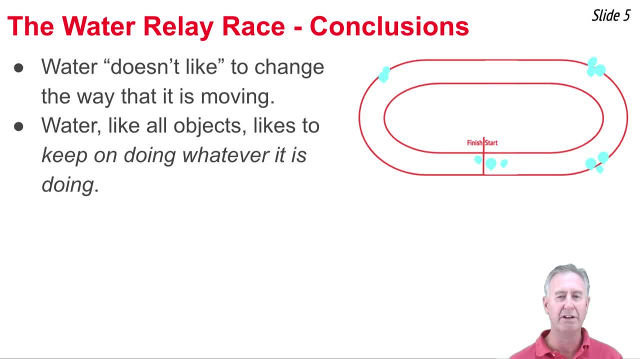 Like all objects, if it's at rest, it wants to stay at rest, And if it's moving, it wants to continue moving in that same speed, in that same direction. Water likes to maintain its so-called state of motion. Water has this thing that we call inertia. 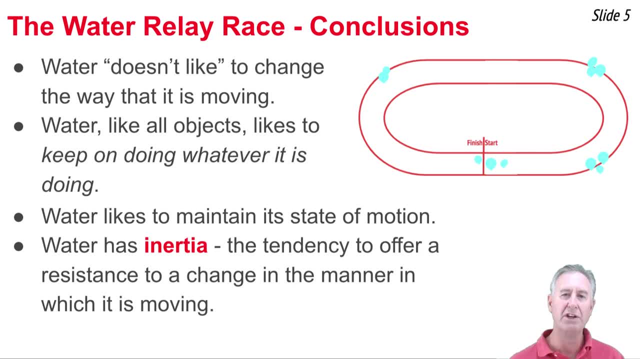 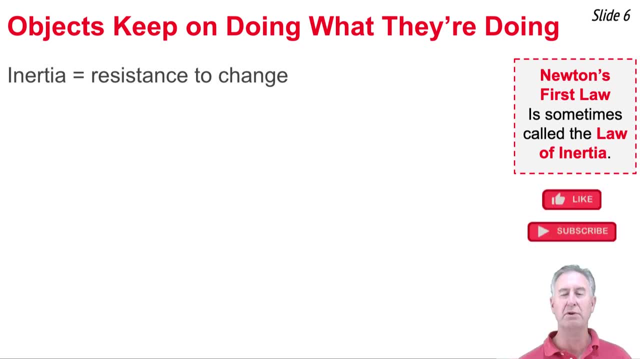 It's a property of the objects that cause them to resist changes in the way that they're moving. Well, this property called inertia is not just true for water. It's true for all objects. All objects want to keep on doing what they're doing. 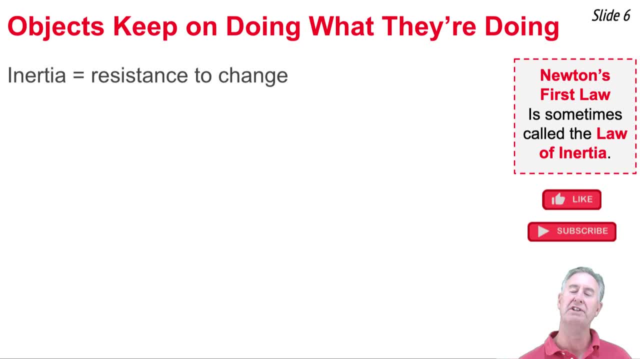 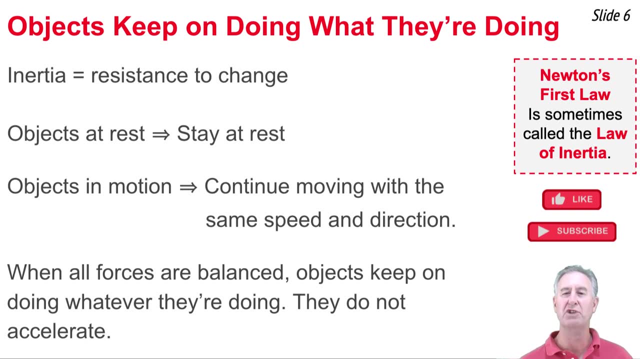 They all possess this property of inertia, The tendency to resist a change in their state of motion. The idea is that objects that are at rest tend to stay at rest. They resist a change from this at rest state, And objects that are moving at two meters per second to the right want to keep moving. 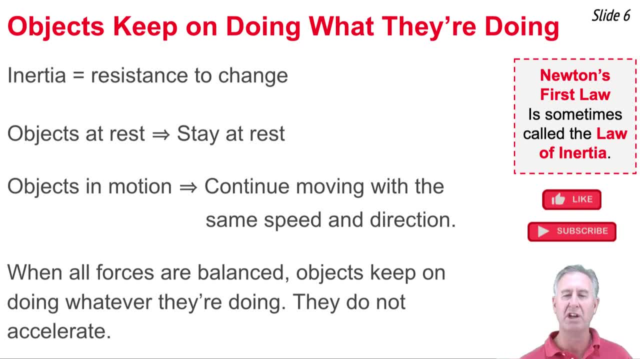 at two meters per second to the right and resist a change in this constant velocity state of motion. When all the individual forces that act upon an object are balanced, objects keep on doing what they're doing. They have inertia, a resistance to a change in the state of motion. 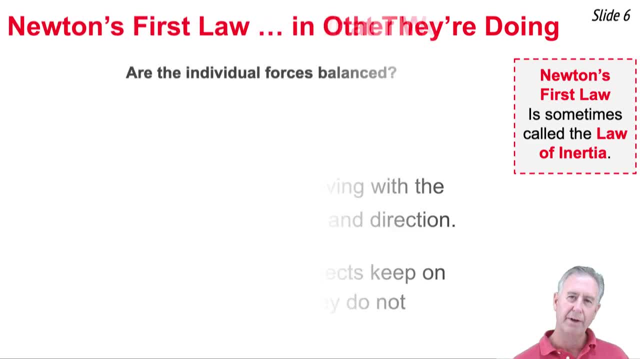 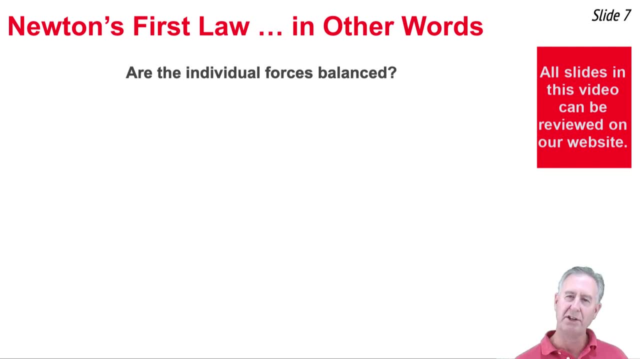 They just simply don't want to accelerate. So we're back to Newton's first law of motion, And here's another way to put it. The first thing you have to do is ask the question: are all the individual forces acting upon the object balance? 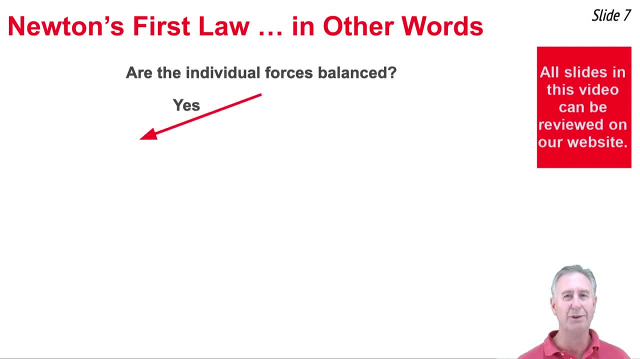 And if the answer to that question is yes, then we're talking Newton's first law of motion, And what we can say is that objects don't accelerate. Their a is equal to zero meters per second squared. Now this, of course, can mean one of two things. 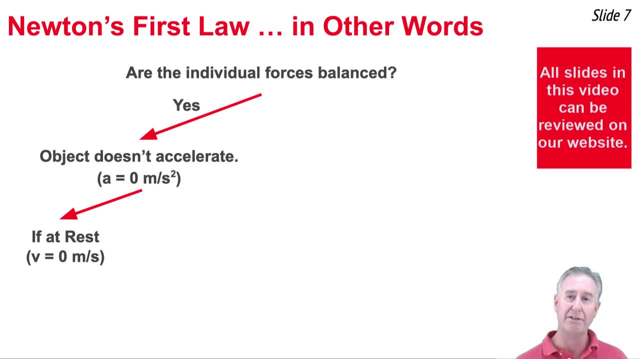 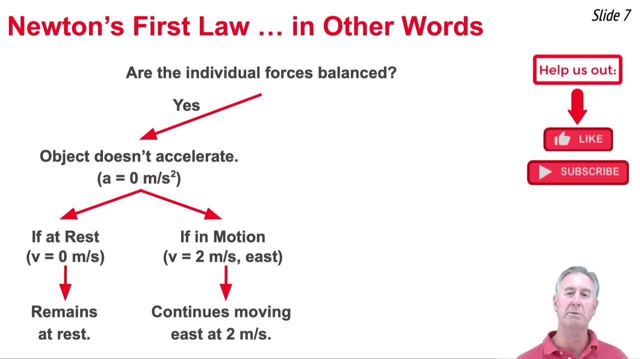 First, it can mean that if the object's at rest, has a velocity of zero meters per second, it's going to stay at rest. Or it can mean that if the object's moving- maybe its v is two meters per second to the east- then it's going to continue moving with that speed of two meters per second in the 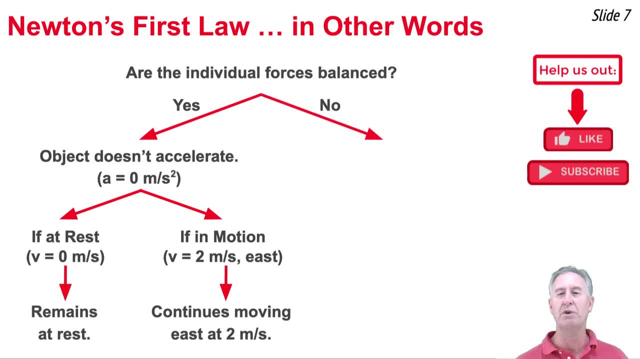 direction of east? If the answer to this original question is no, then we're going to have to move the object to the east. If the answer to this original question is no- the individual forces on the object are not balanced, they're unbalanced- then what we have to conclude is that the objects will 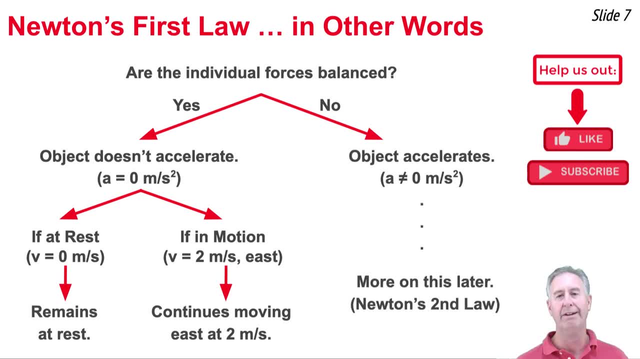 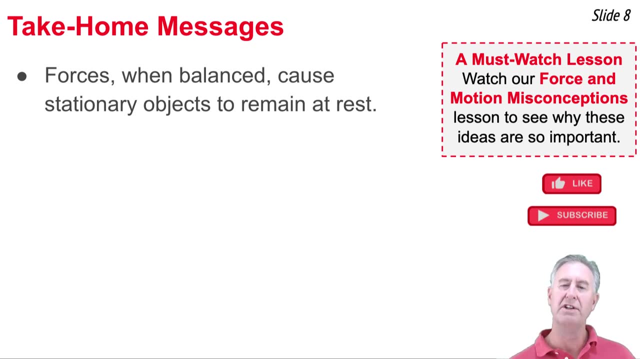 accelerate And the acceleration value? well, we'll talk more about that later, Because that's now Newton's second law of motion. let's not jump ahead of ourselves. So here's some take home messages. First of all, forces, when balanced, cause stationary objects to remain at rest. 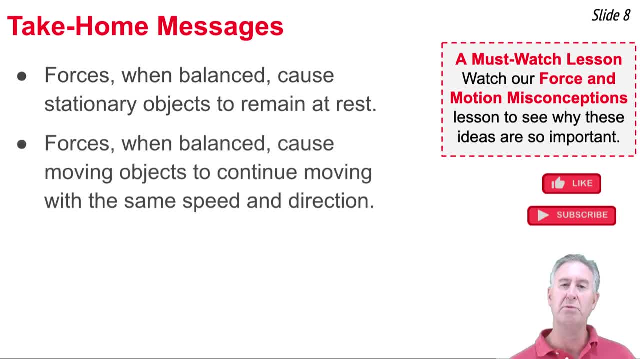 Second, forces when balanced cause moving objects to continue moving with the same speed and in the same direction. Both of these claims could be summarized simply to say: forces when balanced lead to zero acceleration. And our third little bullet point here is that forces when unbalanced cause objects 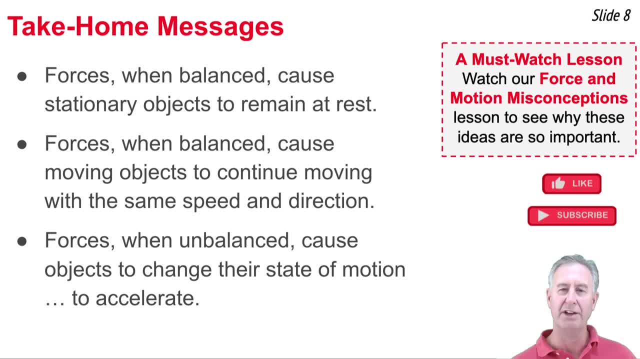 to change their state of motion, Whether moving or at rest. when forces are unbalanced, objects will accelerate. It's at this time, in every video, that I like to give you an answer, An action plan, A way to put this learning into action and sort of make it stick. 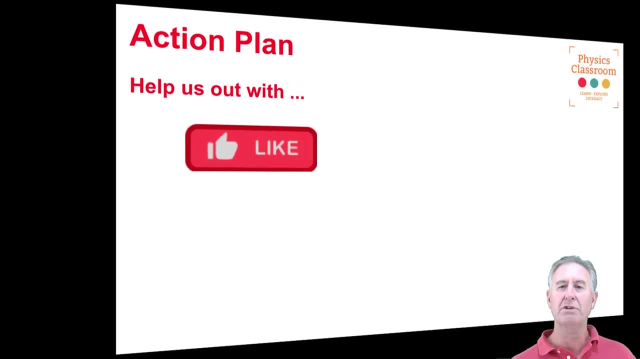 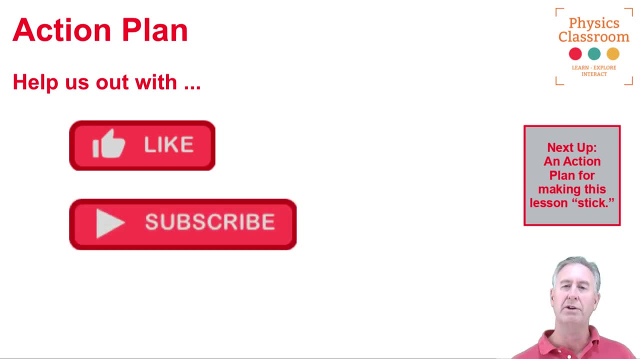 Before I give you that action plan, I'd like to ask a favor of you. First of all. if you liked the video, could you press the like button? If you really liked it, why don't you hit subscribe? Once you subscribe to our channel, why don't you tap on the bell and get notifications?